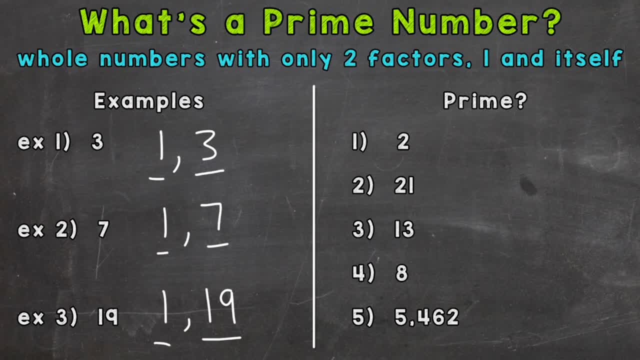 One and the number itself. So let's take a look at five other examples and see if they are prime or not prime. So let's take a look at number one on the right-hand side of the screen, where we have two. Now, two is a very unique number and we'll see why here in a second. 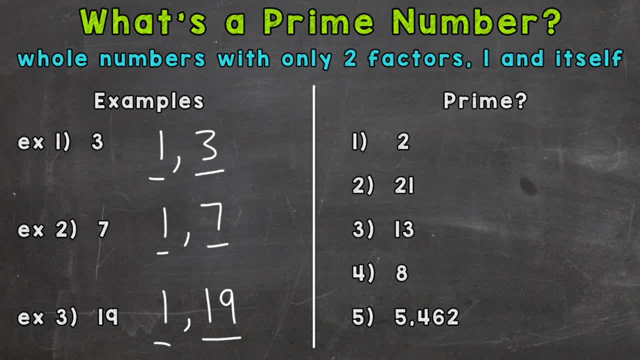 So let's think of the factors of two, the numbers that go into two. Well, it's only one, and two So one, and the number itself, two So two, is a prime number And it's unique because it's the only even number that's prime. 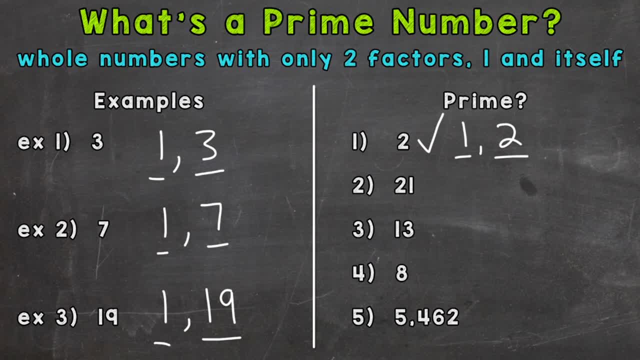 Any other even number is automatically not prime. So let's take a look at number two, where we have twenty-one. So let's think of the factors or multiplication facts that equal 21 or the numbers that go into 21.. However, it works best as far as you're thinking and coming up with factors. 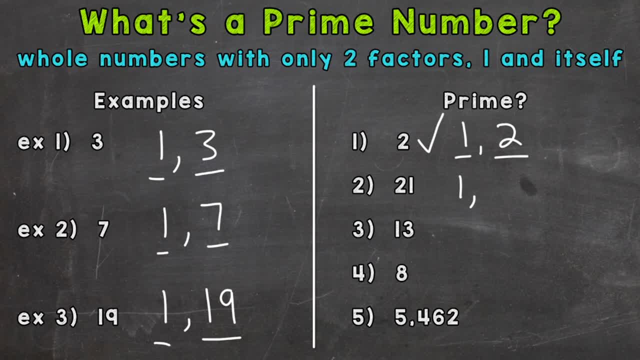 So we know that 1 times 21 equals 21.. So 1 and 21 are factors, but also 3 and 7. And I'll add 21 to the end there. So 21 has more than two factors, more than one in itself. 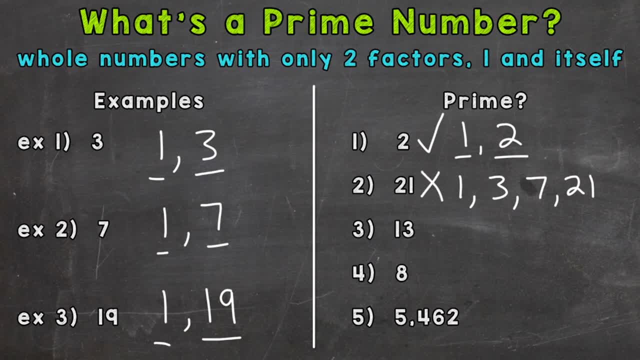 So 21 is not prime. It's considered a composite number And I actually have a video about composite numbers where I go into more detail. I'll drop that down in the description On to number 3, where we have 13.. 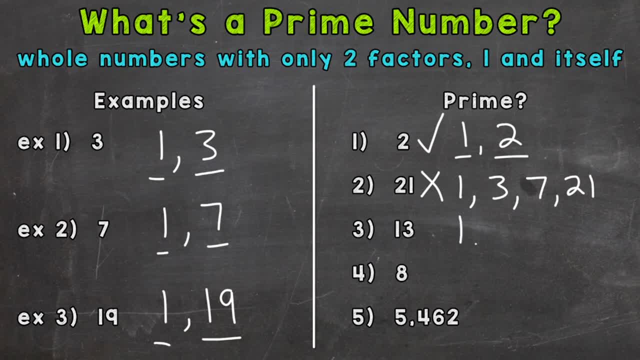 So the only factors of 13 are 1 and 13.. So 1 and the number 13 itself. So 13 is prime. Next we have 8.. So we know 1 and 8 are factors, But also 2 and 4 can go into 8.. 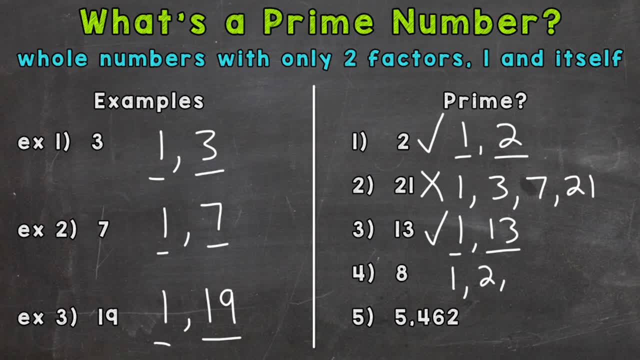 2 times 4 equals 8, so 2 and 4 are factors, So we have more than two factors there. So 8 is composite, It is not prime. And lastly, number 5, we have 5462. 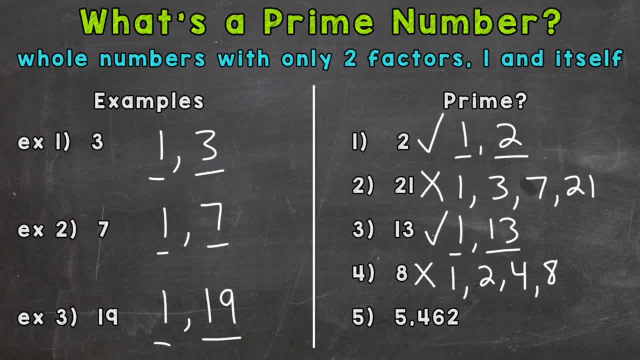 Now we do not want to write out all of the factors for that number to determine if it's prime or not. We can automatically tell because, like we mentioned earlier, mentioned earlier, all even numbers except two are composite. They are not prime because we know.